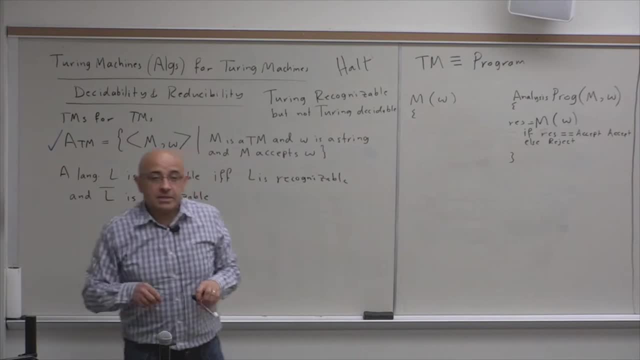 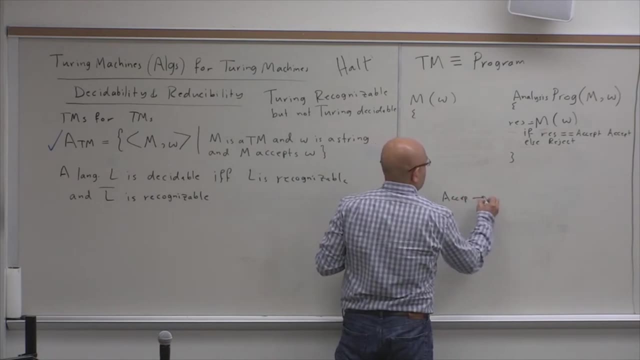 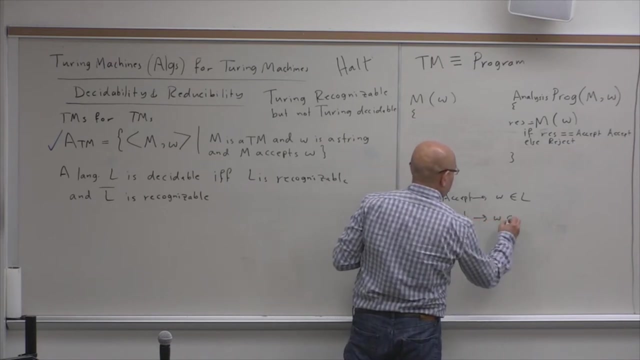 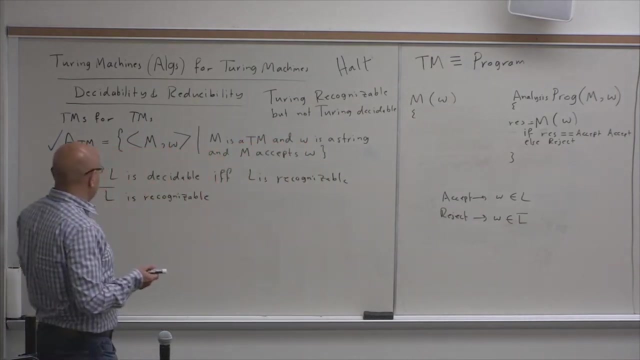 we know that this will terminate right, Because it's, you know, if it's accept. accept means belongs to L Accept means W belongs to L. Reject means W belongs to L complement. Now, last time we said that, if we know that both the language 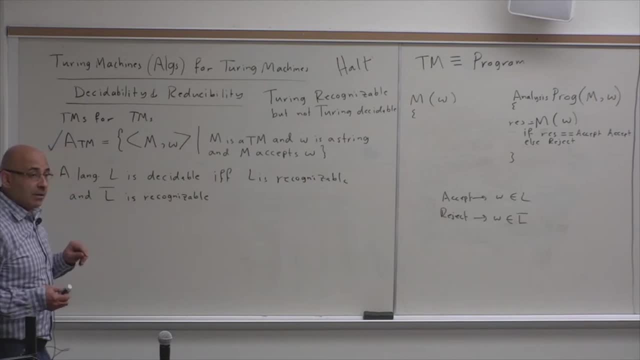 and its complement are recognizable, then we can build a decider for that language. because as soon- Assume that you know, you have, you know m for the language and you have m bar for the complement of the language, You can run both m and m bar in parallel and one. 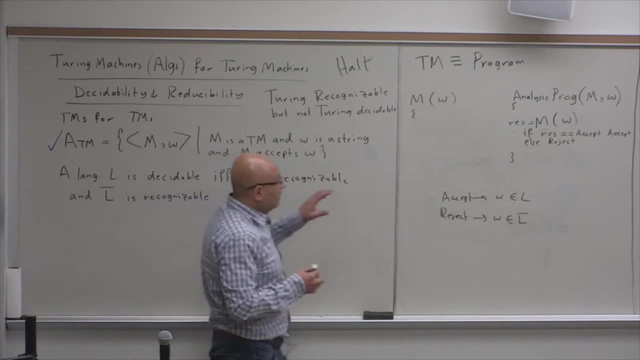 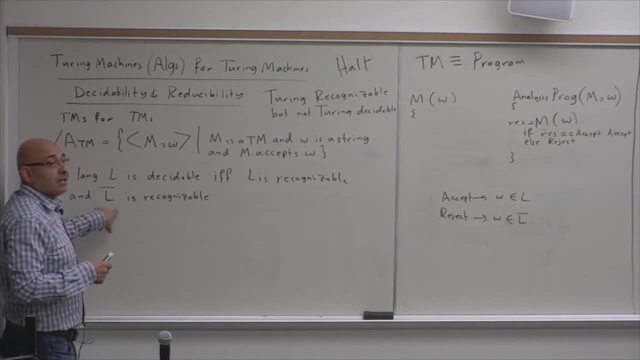 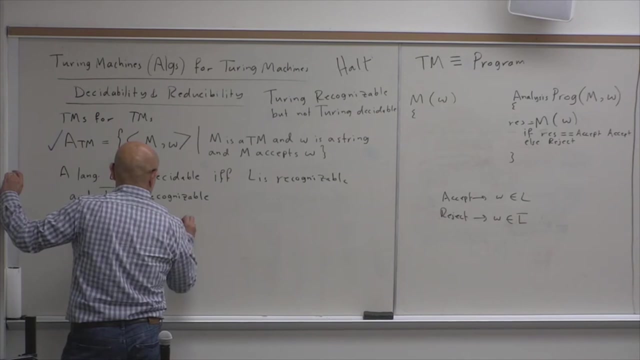 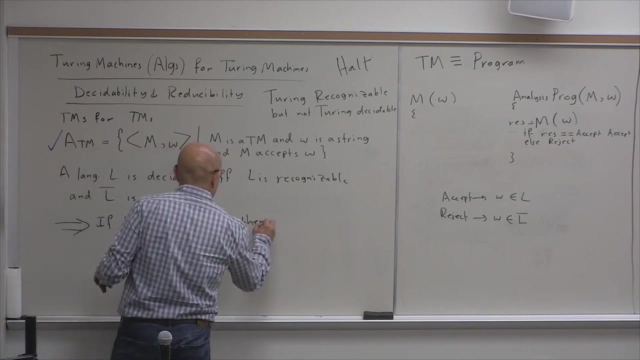 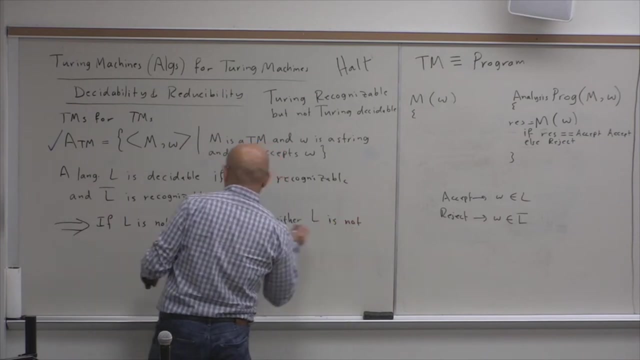 of them is going to accept. But in fact, you know, the fact that this problem is not decidable means that the complement of this language cannot be recognizable. So, if you know, this implies that if l is not decidable or undecidable, then either l is not recognizable. 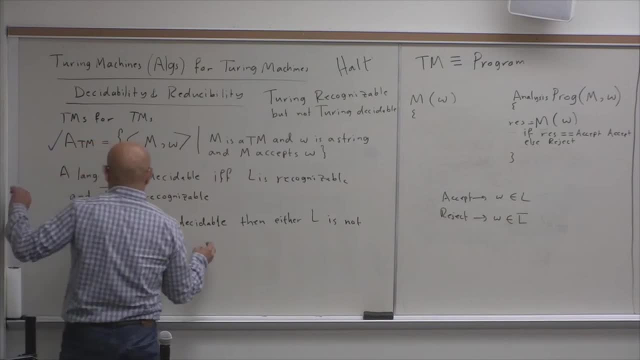 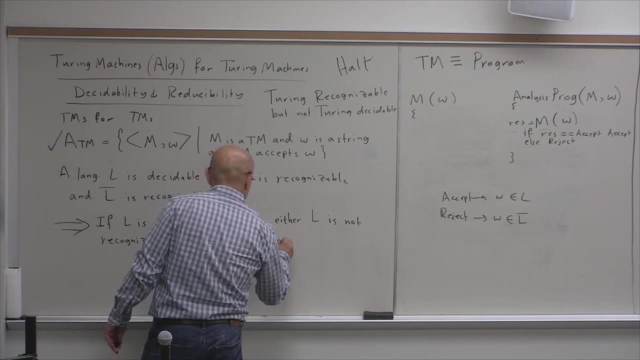 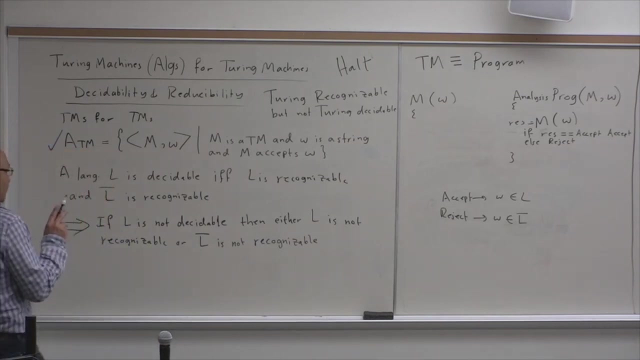 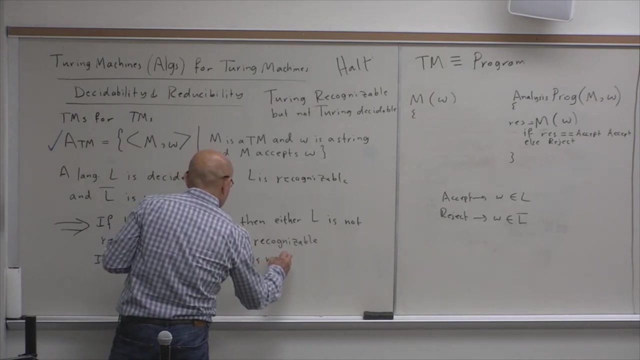 or it is not recognizable, Or l complement is not recognizable. So if l is not decidable, then either l is not recognizable, or l prime or l complement is not recognizable. And if l is not decidable and L is recognizable, what can you say about L prime? 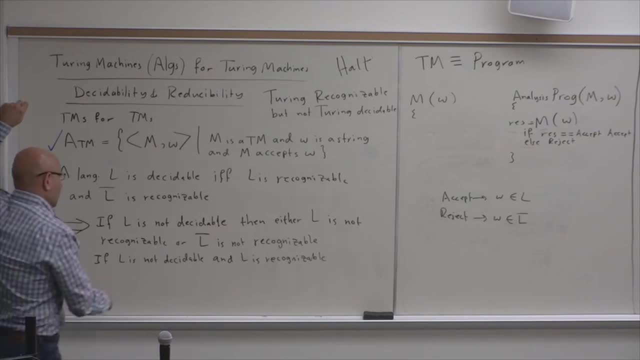 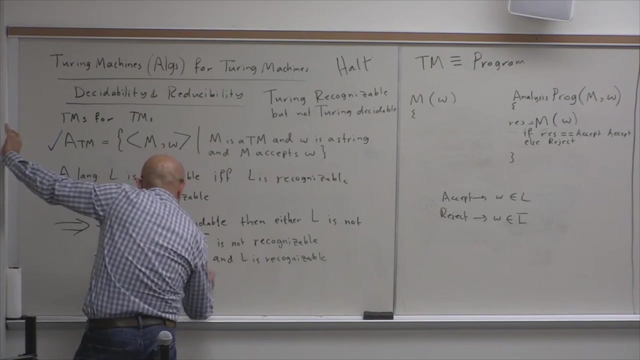 If L is not decidable or undecidable and L is recognizable, what can you say about L bar The complement? It's not recognizable. It's not recognizable. Yeah, it cannot be recognizable. Okay, Then L prime is not recognizable. 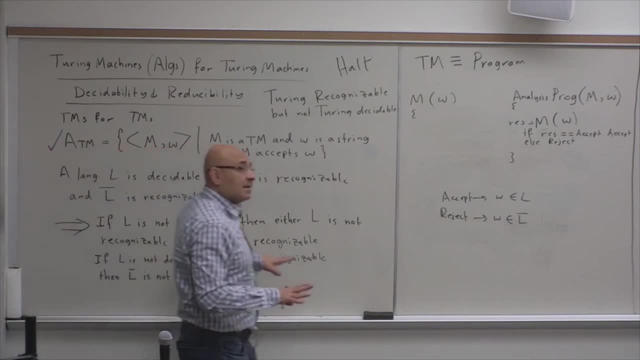 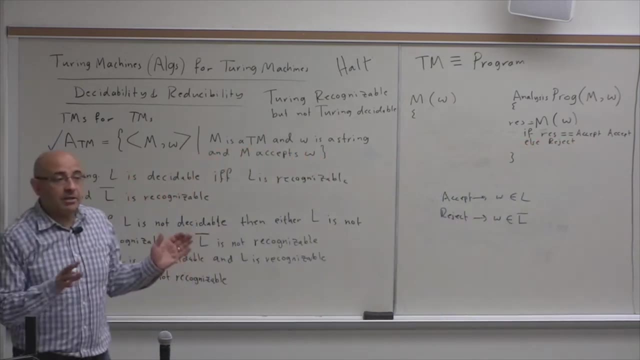 Okay, So if a language is not decidable, then either the language and its complement or both unrecognizable, or at least one of them is unrecognizable, As we said last time, if both the language and its complement are recognizable. 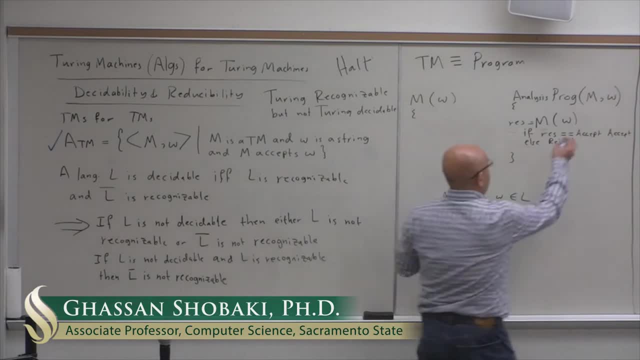 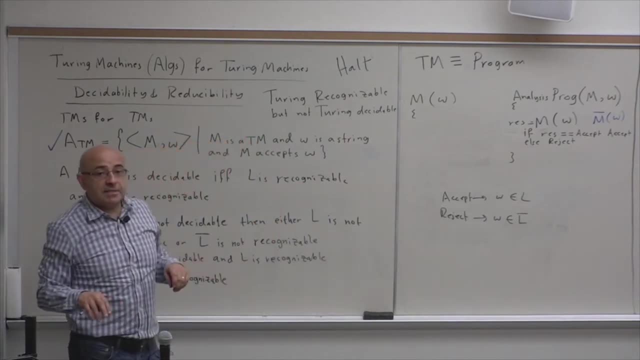 then we can run them in parallel. So here you know, we can run M and M bar of W in parallel, And if one of them accepts, then we know what the result is. If M accepts, then we accept, If M. 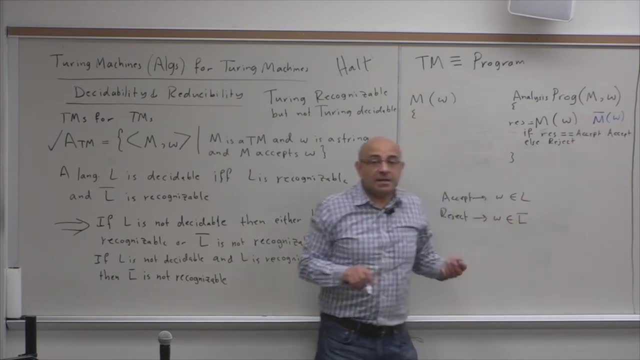 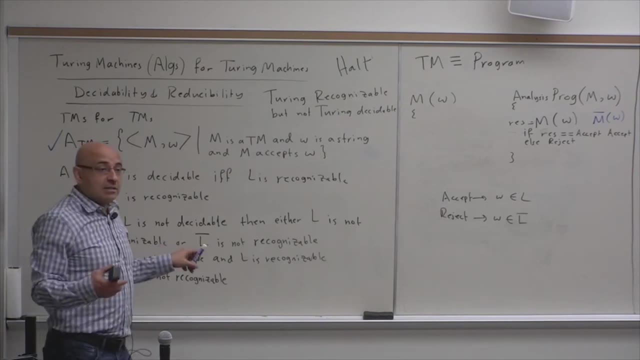 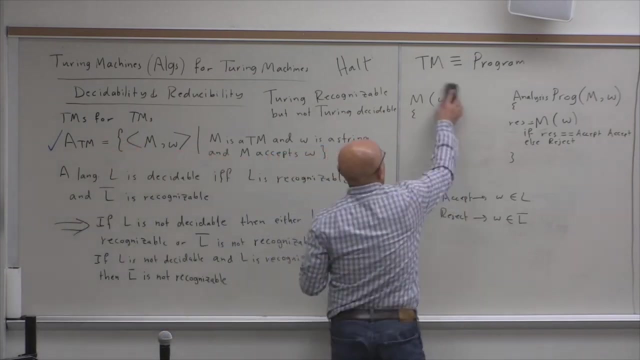 Bar or the complement of M accepts, then we reject. Okay, Any questions on this. Now there is an interesting argument that Turing machines cannot recognize all languages, or that the number of languages is greater than the number of Turing machines. 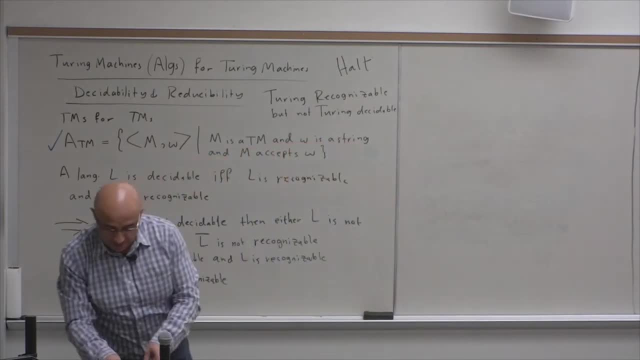 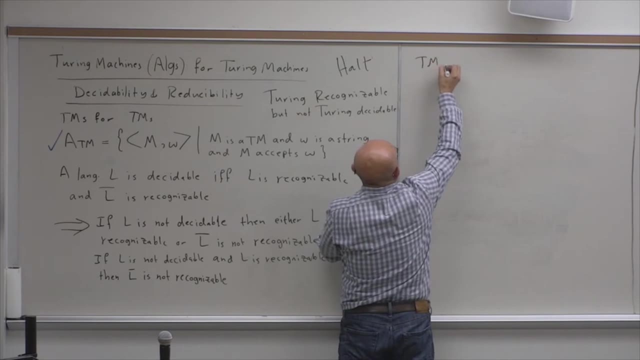 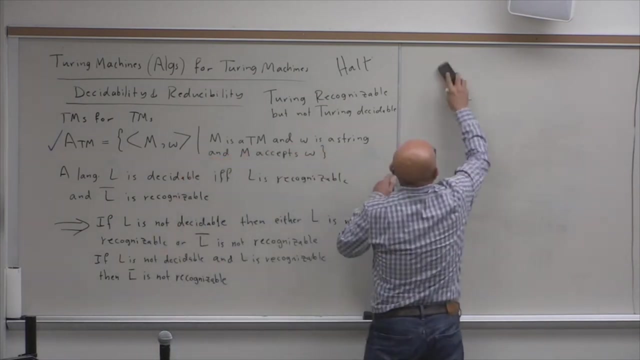 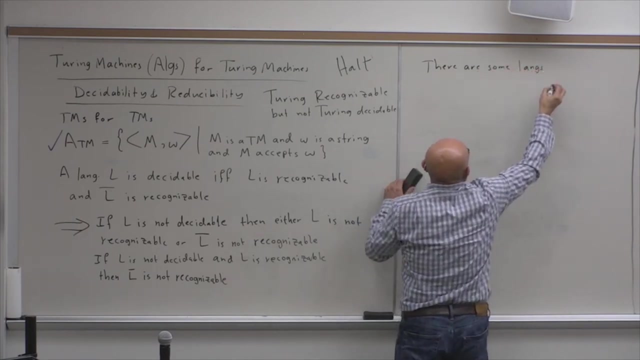 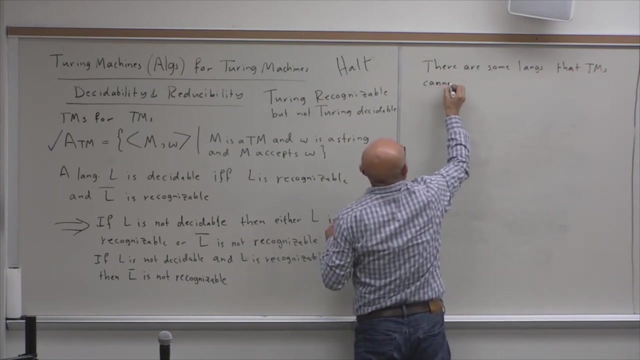 Okay, So again, this is something that I will explain intuitively. So Turing machines cannot, or let's. there are some languages that Turing machines cannot recognize or for which there are no Turing machines that recognize, that are not recognizable by Turing machines. 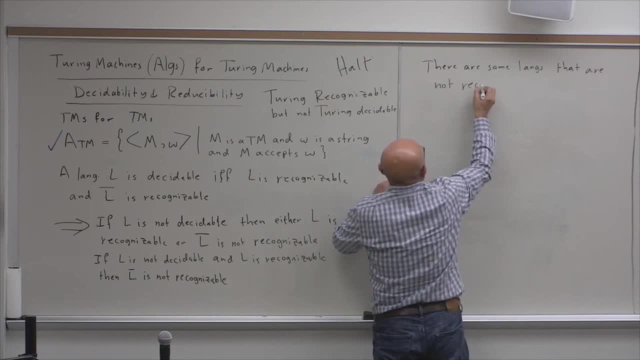 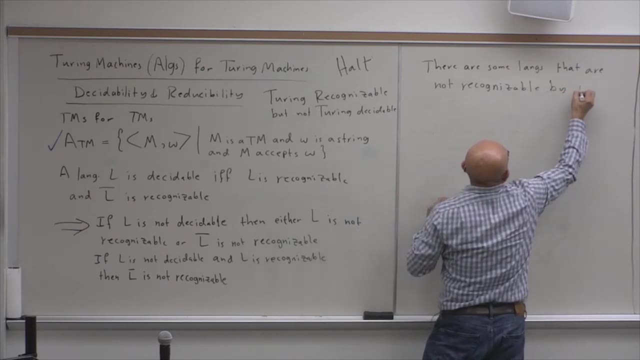 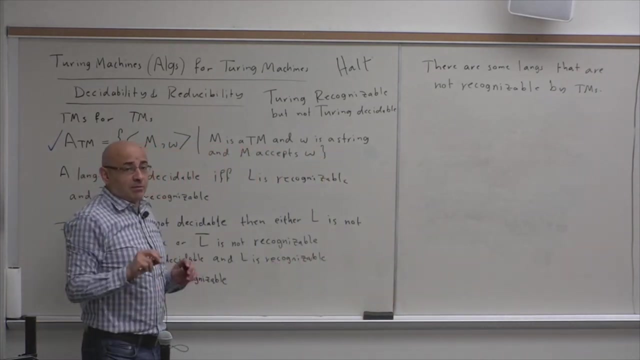 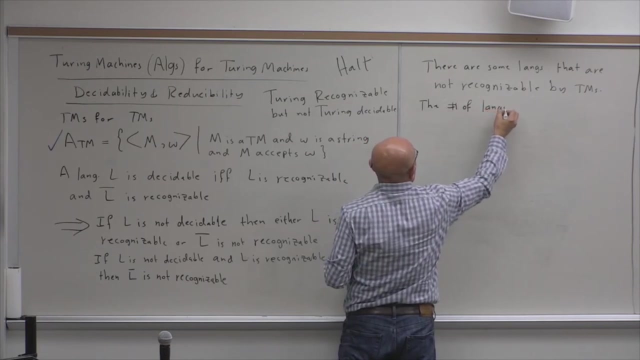 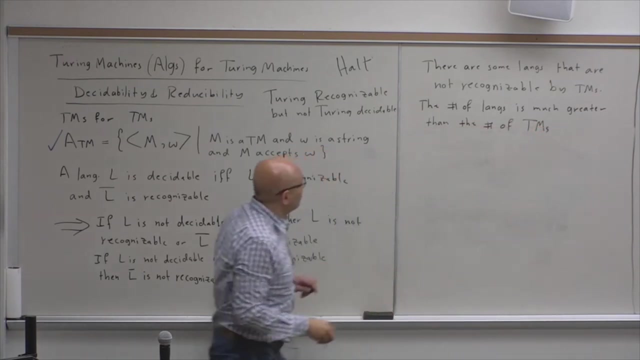 that are not recognizable by Turing machines. And why? Because Because the number of languages is much greater than the number of Turing machines. The number of languages is much greater than the number of Turing machines. Why? So let me show to you. 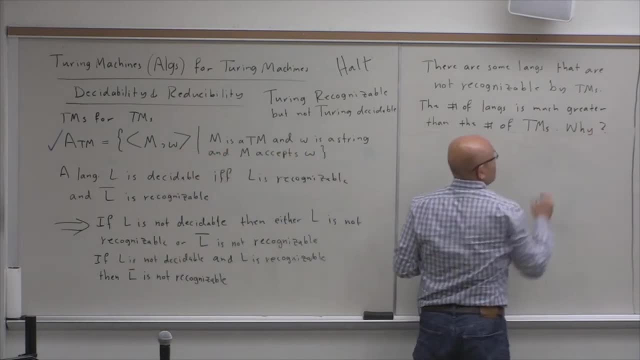 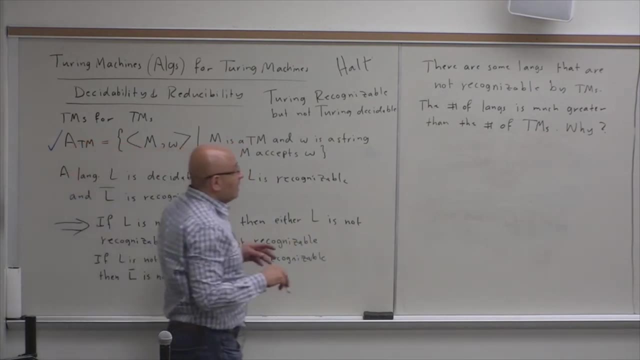 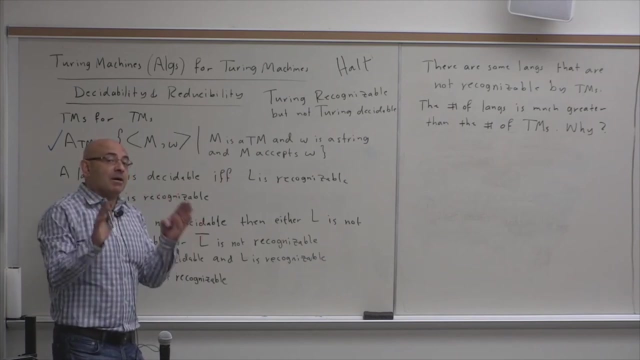 Because a Turing machine, the Turing machine itself, a Turing machine is a program And a program is a string, And the number of strings is limited for a given alphabet is limited by the number of elements in sigma star. So or is bounded by: 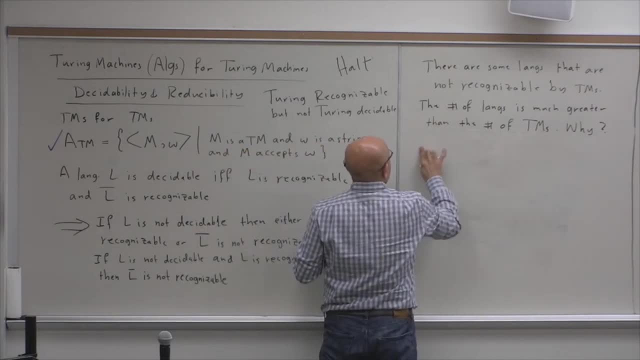 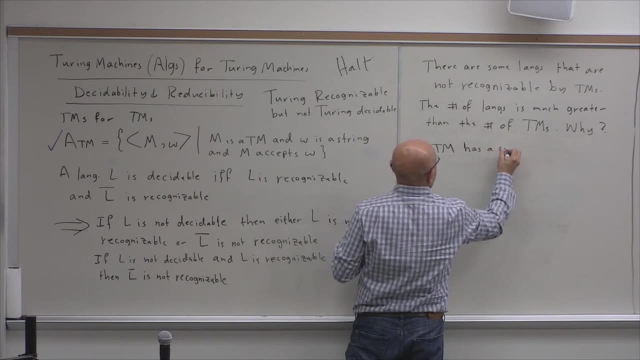 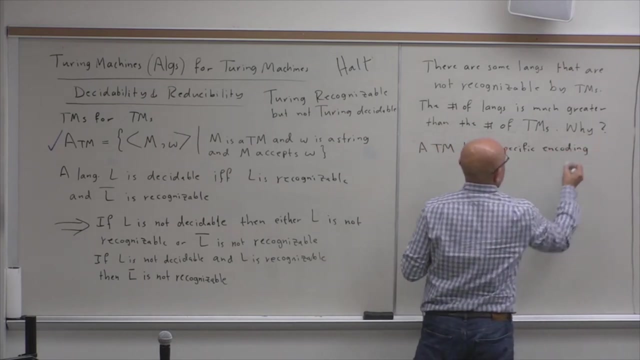 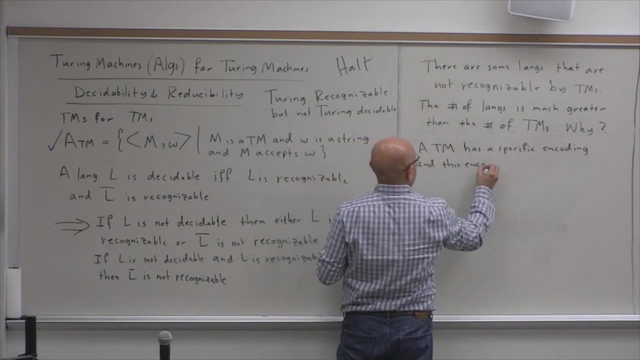 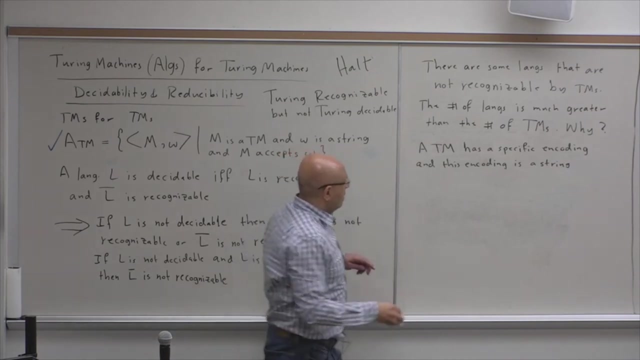 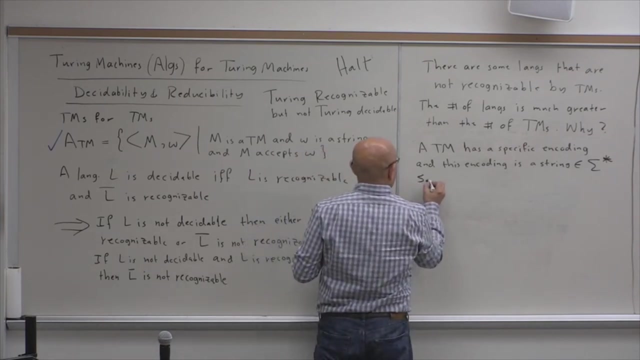 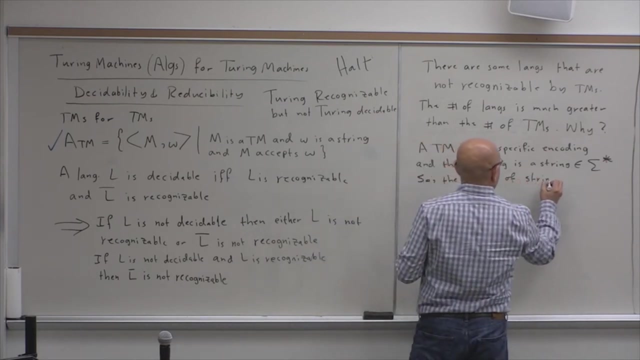 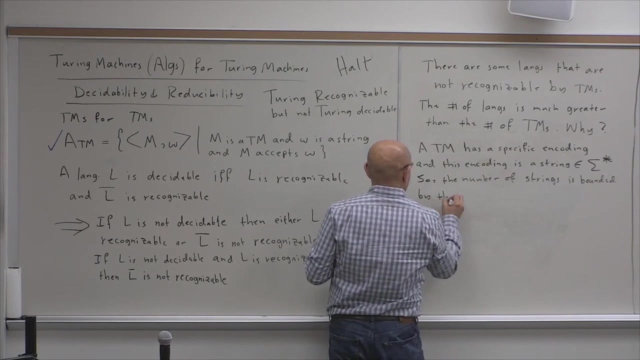 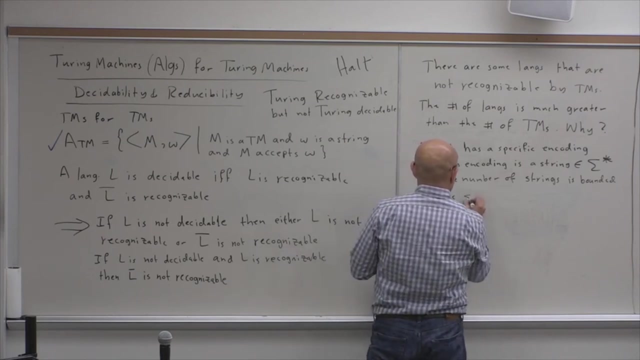 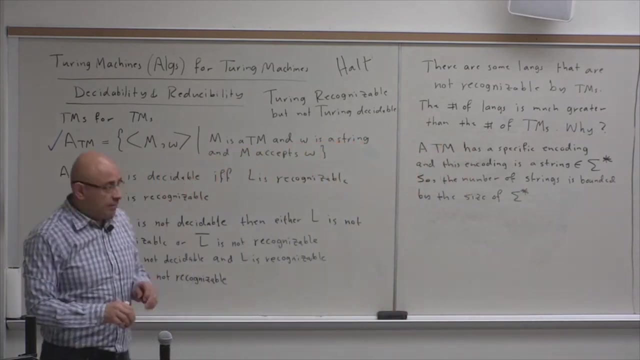 So the a Turing machine has a specific encoding, And this encoding is a string That belongs to sigma star. So the number of strings is bounded by the number or the size of sigma star. Okay, so now let's show intuitively why there are more. 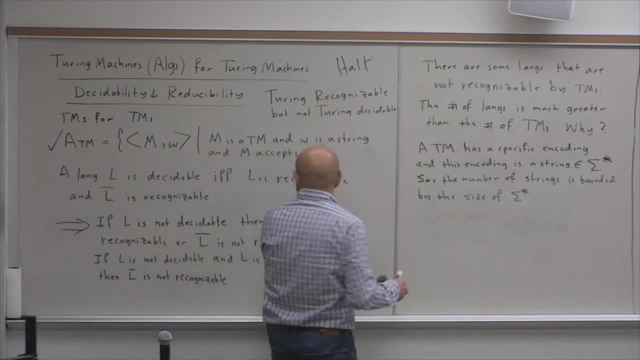 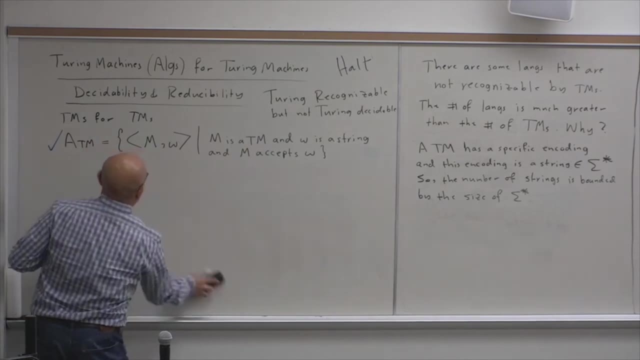 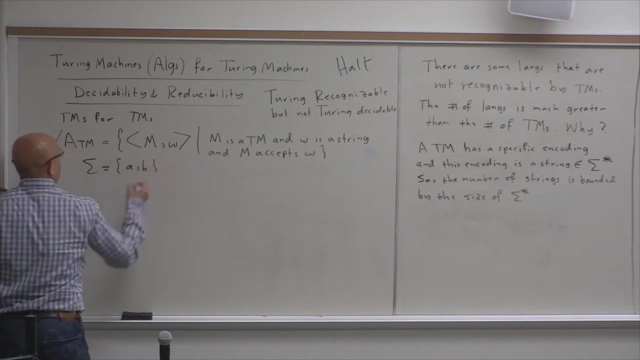 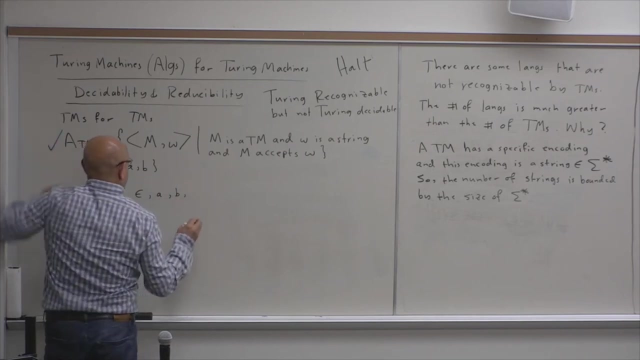 languages than there are strings. So if we you know, if your sigma is AB, your sigma star is going to be this: The set of all strings, The set of all strings is going to have epsilon, Then it's going to have string A, string B, Then the strings. 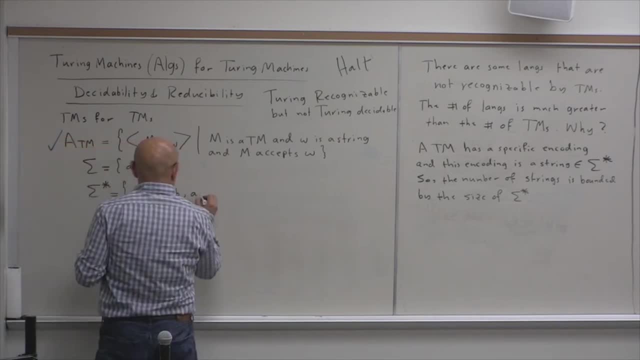 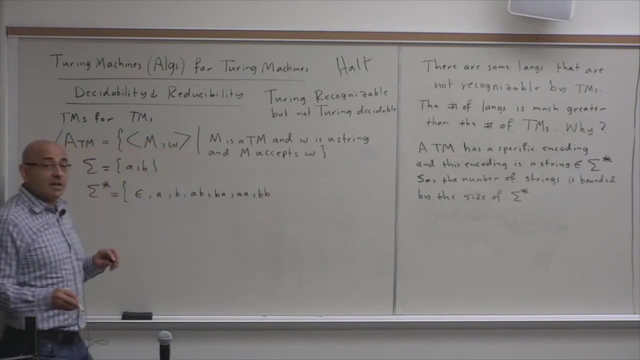 of length two: AB, BA, AA, BB. So these are all the strings of size two. Then you'll have the strings of size three, And then you'll have the strings of size three, A, A, A, A, A, B, etc. So these are the strings of size 0. 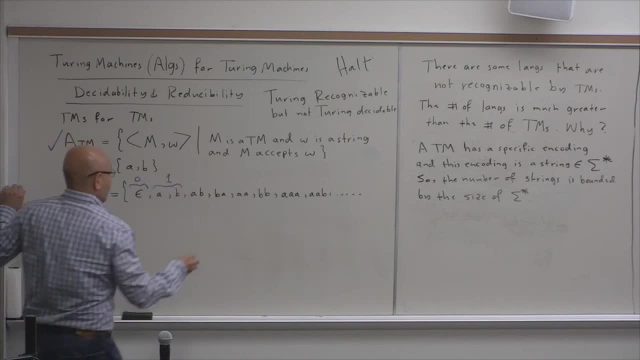 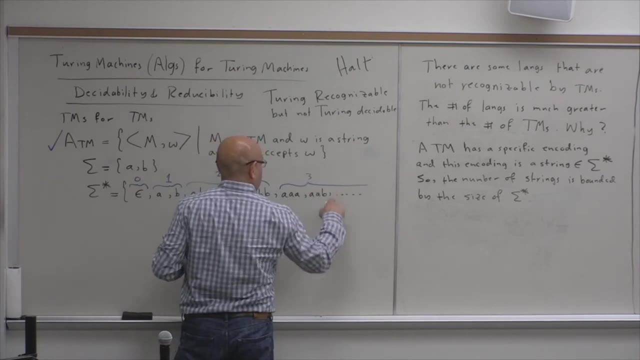 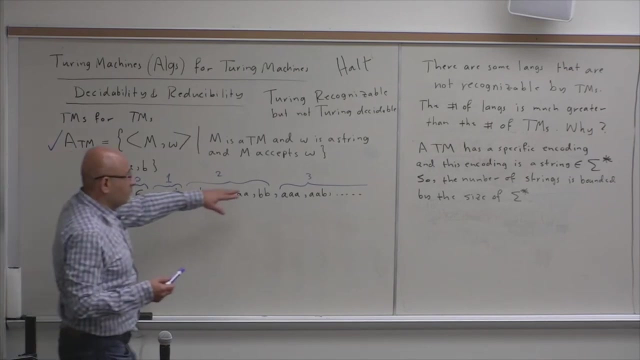 Then the strings of size 1., Then the strings of size 2. And then the strings of size 3, but this is not all of them. So this is, sigma star, what it looks like Now when we look at the set of languages. a language is what. 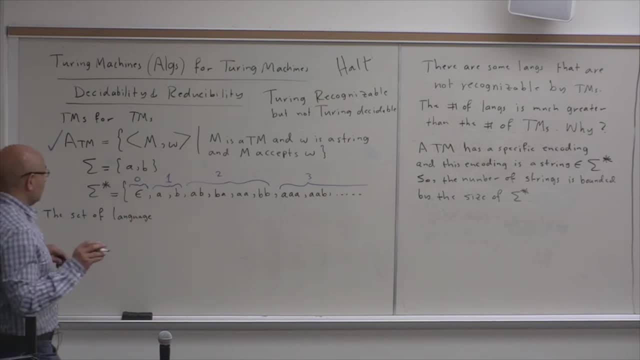 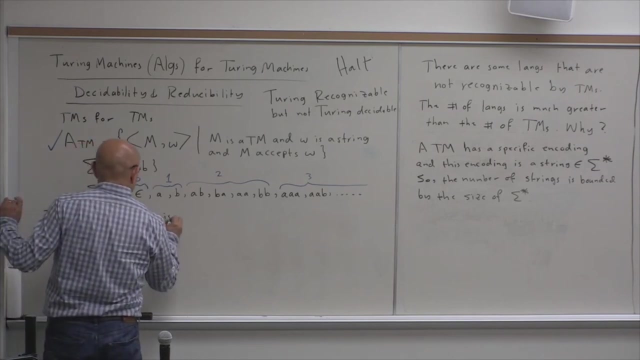 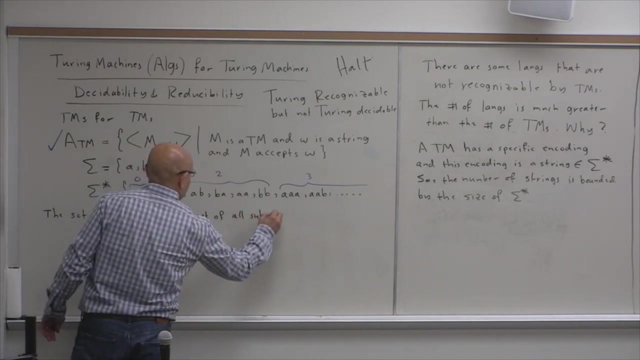 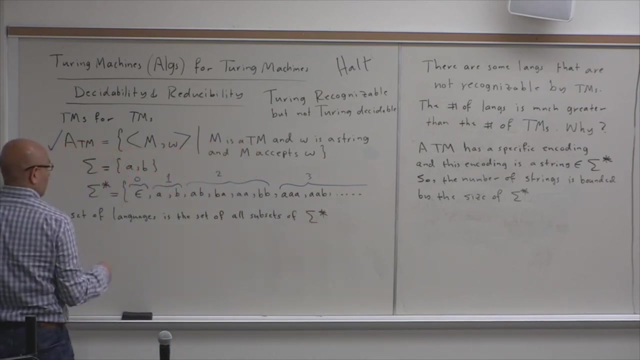 A language is a subset of the strings in sigma star. So the set of languages, in fact, is the power set of sigma star. The set of languages is the set of all subsets of sigma star, So let's call it L? LO. 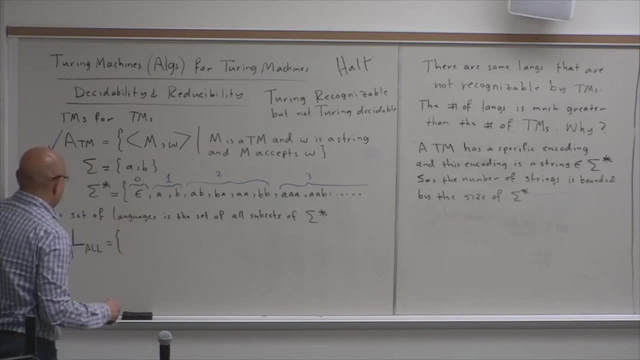 Set of languages, Set of languages, Set of languages. So this is going to have in it the set of the strings, that well, it's going to have the empty language, Then the language that has an empty string in it, one string in it. 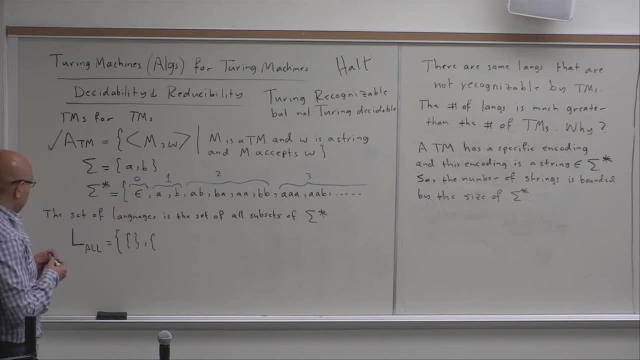 But the language that has one string in it is going to have. well, let's look first at this. Only this part of sigma star, Only this, So you will have. for these strings you will have. the set of all languages is going to have A by itself. 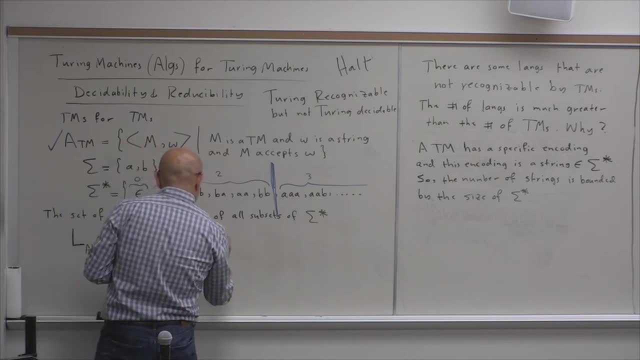 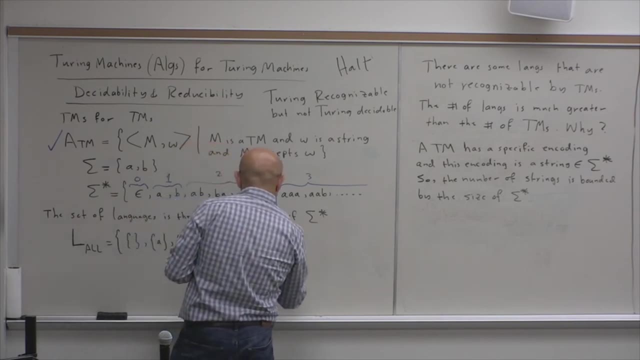 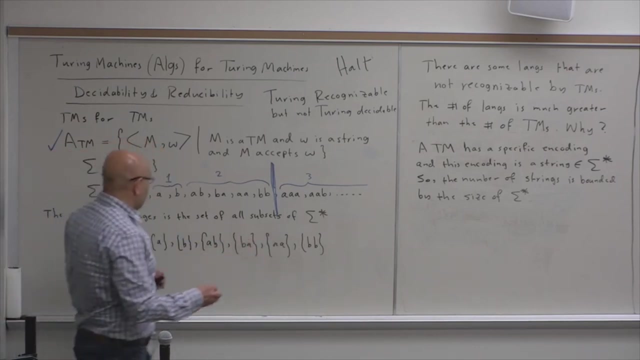 B by itself, AB by itself, BA by itself, Right, AA by itself And BB by itself. So all the strings by themselves, Then the set of languages that have two strings. So you will have, you know, epsilon and A, Then epsilon and B. 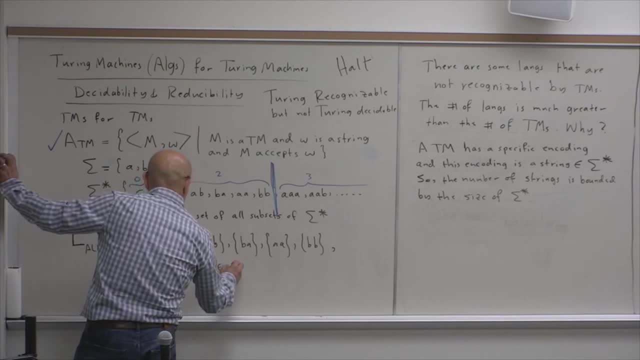 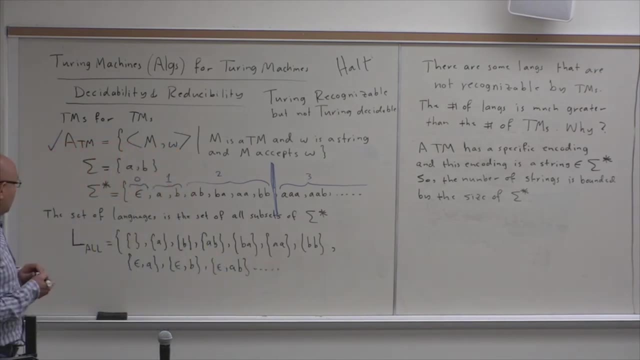 Epsilon and AA or AB, Right Right Now. does this convince you that the set of languages has more elements in it than the set of strings? So, in fact, for this part, you know, for this part of sigma star, you have like four, seven elements. 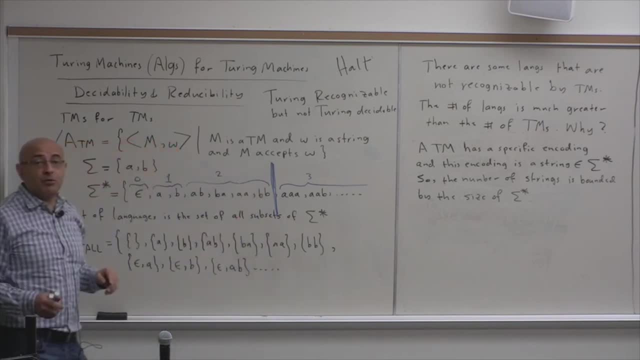 The power set that corresponds to only this, is going to have two power seven in it. It's going to have two power seven languages. So for seven strings you get two power seven languages, Because each language is going to be, you know, is either take. 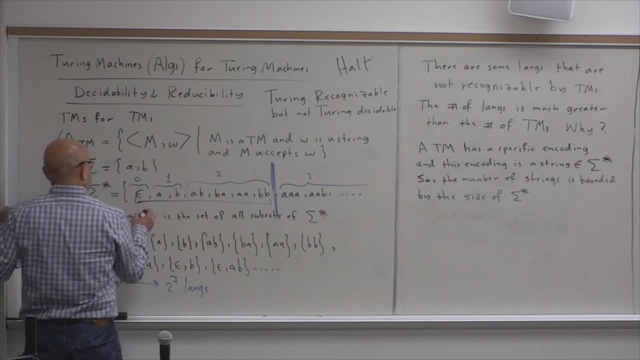 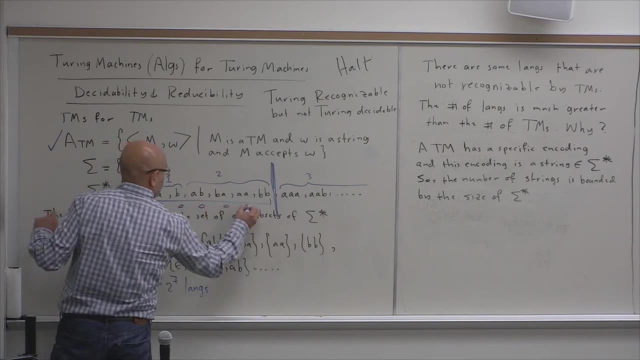 or not take one of these strings. It's like you know, if you say this one, one, I'm going to take epsilon and one Epsilon and A, I'm not going to take this, this, this. So there is like a, you know, for each string. 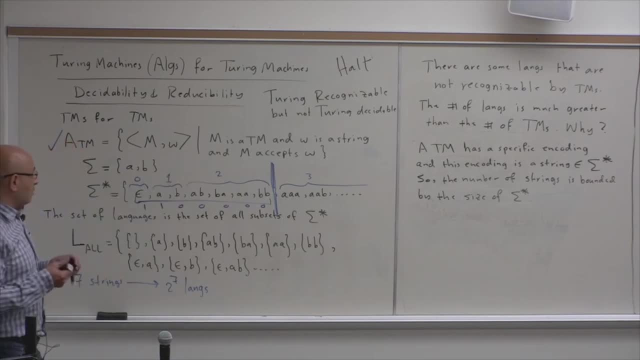 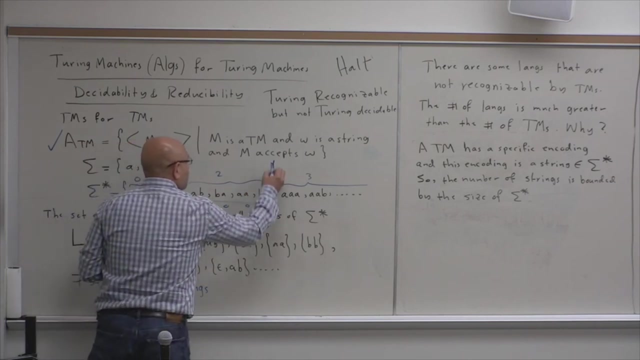 in this language, you determine, you decide whether to take it or not, And there are seven of them And for each one of them there are two possibilities: either take or not take. Then you have two power: seven languages that correspond to only this part. 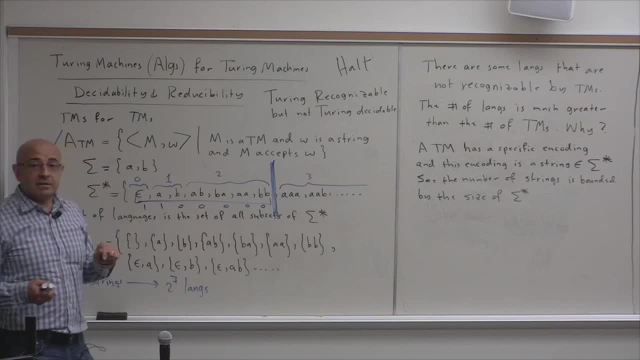 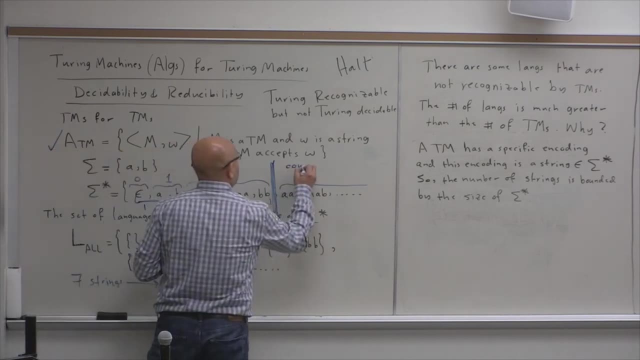 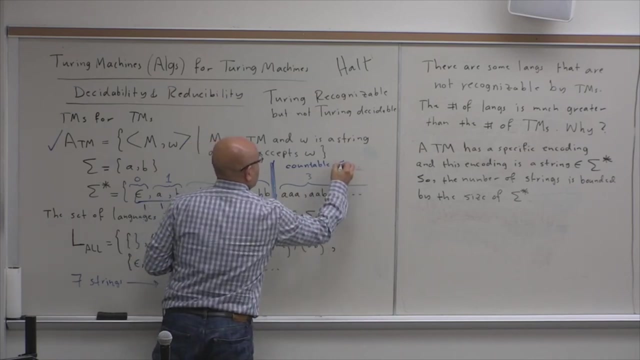 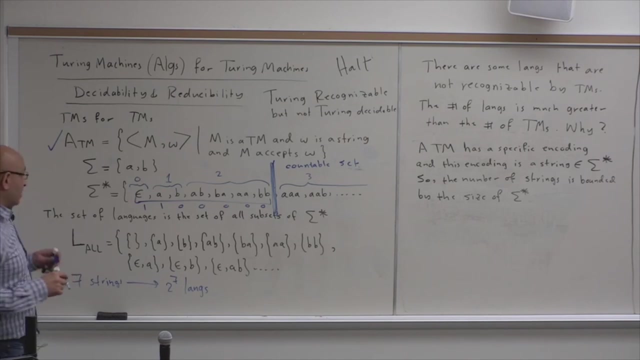 This part of the sigma star. Okay, In fact, you know, we can say that. you know, sigma star is a countable language, is a countable set. A countable set is a set that can be mapped into the set of natural numbers. 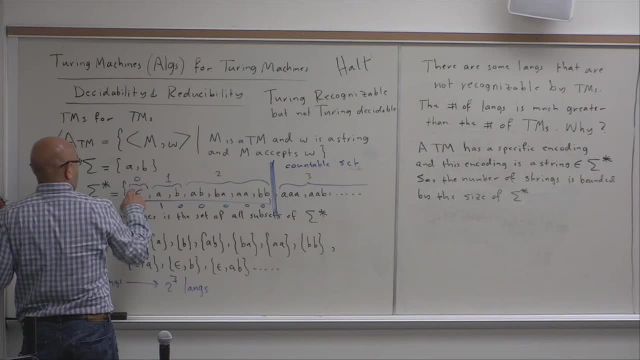 So we can say that you know, this is number one, two, three, four, five, six, seven, et cetera. But such a mapping to the set of natural numbers cannot exist for the set of languages, which is the power set of the set of strings.